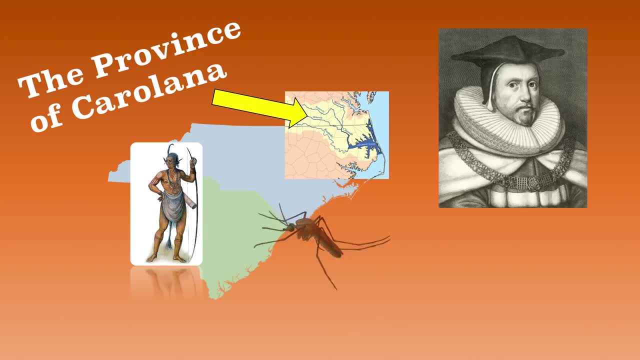 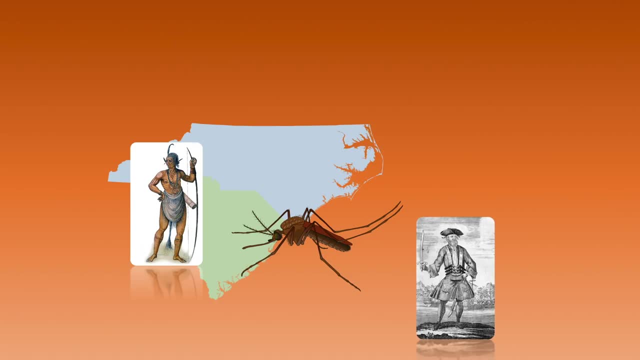 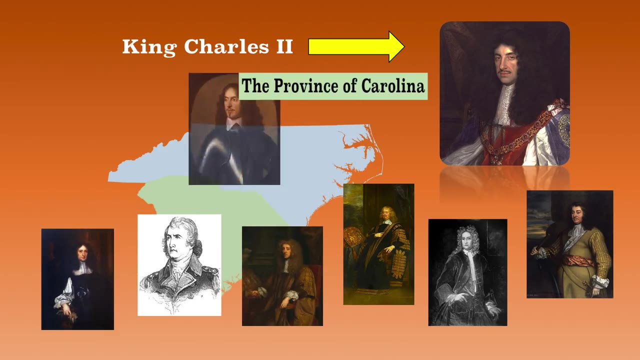 But due to hostile natives, the malaria in smallpox and crazy pirates like Blackbeard going up and down the coast, Heath never colonized the area. Later, King Charles II let eight rich English dudes take over what was now called the province of Carolina to repay them for helping him become king. 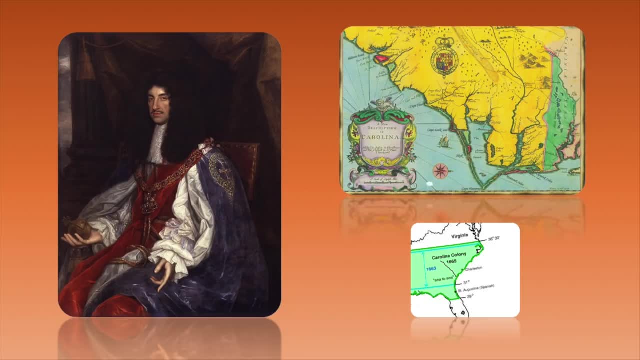 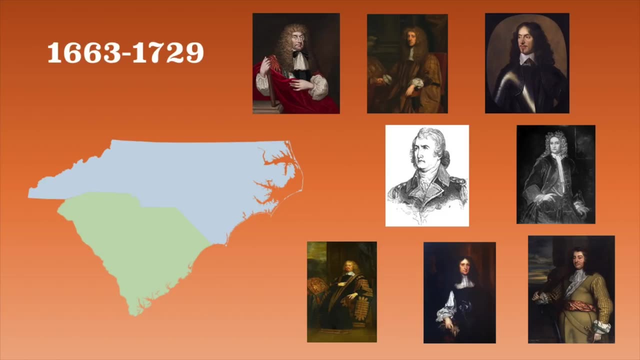 King Charles II wanted the area as a buffer zone between the colonies of the North and Spanish Florida to the South. So when these eight dudes controlled Carolina between 1663 and 1729, they constantly fought and had a hard time controlling the giant area anyway. 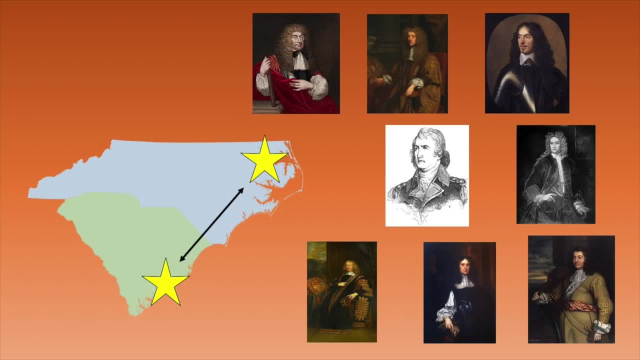 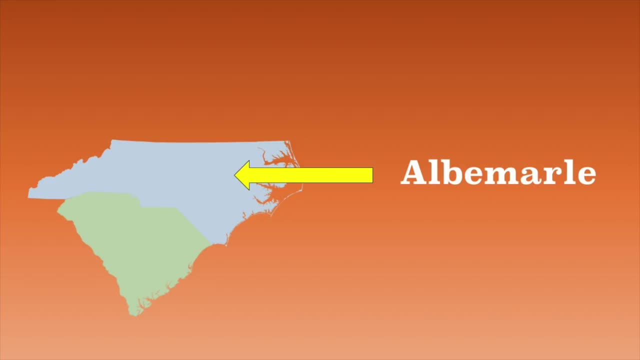 The settlements in the North were so far away from the settlements of the South. after all, In 1669, Carolina became two provinces to try to solve this: The Albemarle Province in the North and Clarendon Province in the south. 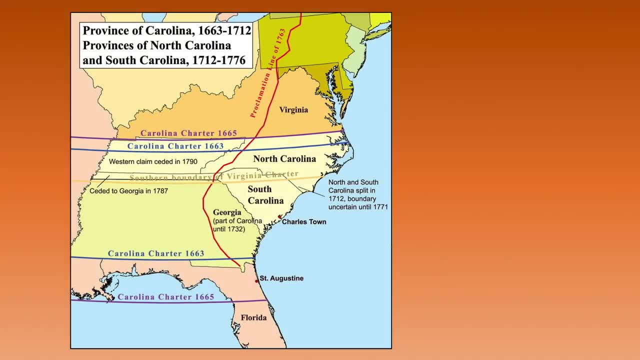 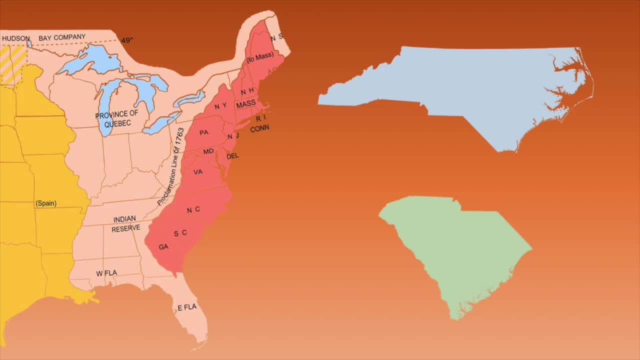 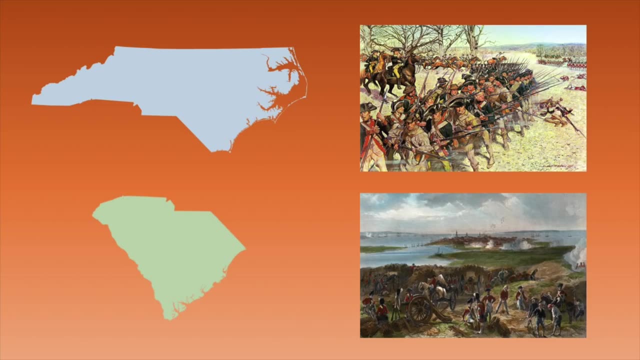 In 1712, they just went ahead and became two separate colonies. But really, historically the colonies have had much more in common than they have had differences. Both were two of the original 13 colonies and both did not hesitate to rebel against the British during the American Revolution after Britain started taxing the heck out of them. 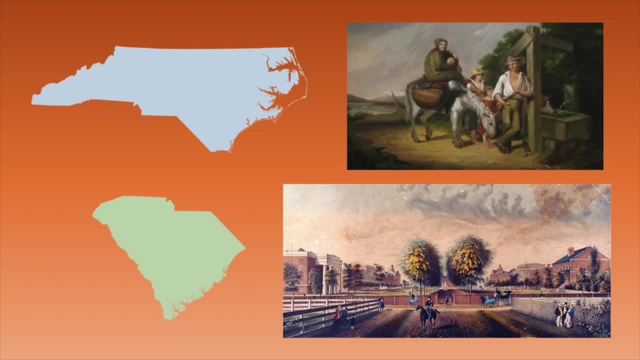 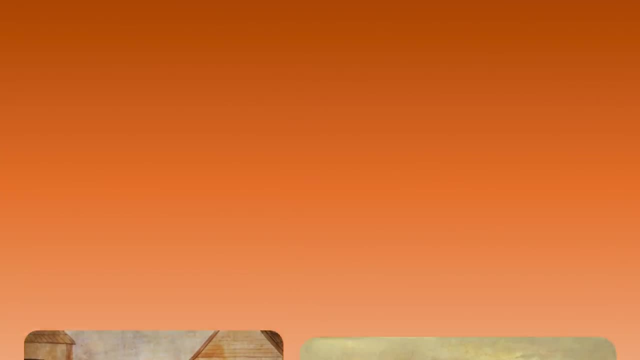 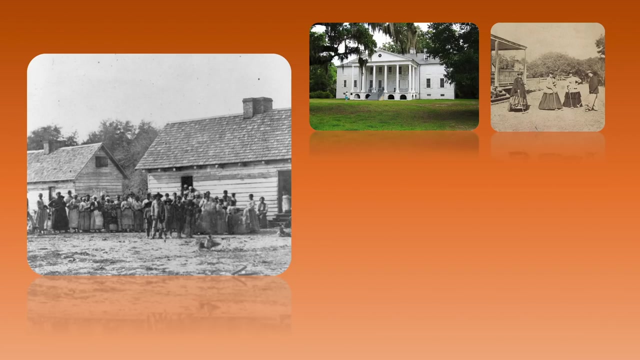 Both remained mostly rural after becoming states relying on agriculture to drive their economies, And that agriculture relied heavily on slave labor. This slave labor helped several planters in the eastern lowland areas of both states to become filthy rich, as they produced lots of indigo rice, tobacco and especially cotton. 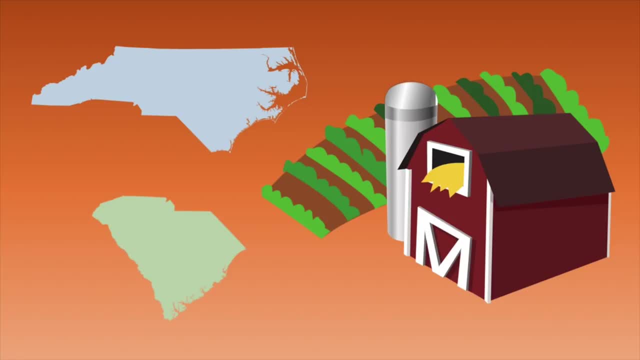 More than half of farmers in both states, however, did not own slaves and were self-sufficient. They had small farms, and the ones who struggled the most tended to be in the west, towards the mountains, During the Civil War, of course. 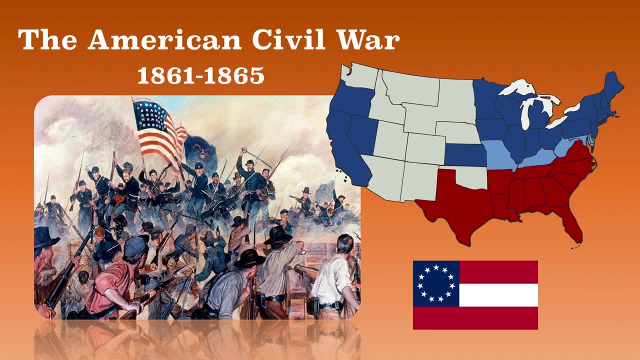 both North and South America were in the middle of the war During the Civil War. of course, both North and South America were in the middle of the war, and both North and South America were in the middle of the war. Both South and South Carolina seceded from the Union and joined the Confederate States of America, but South Carolina was the very first state of all of them to secede. 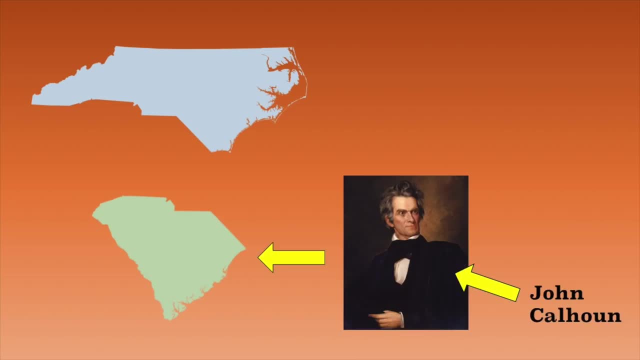 Also, for decades, South Carolina had leaders like John Calhoun who were much more outspoken about seceding and just talked a lot of trash in general about the North and them wanting to take away states' rights, ie slavery. 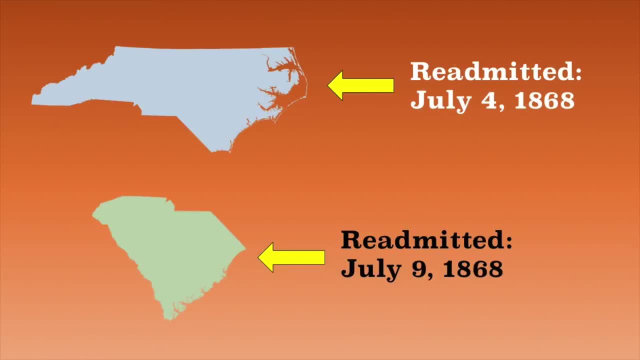 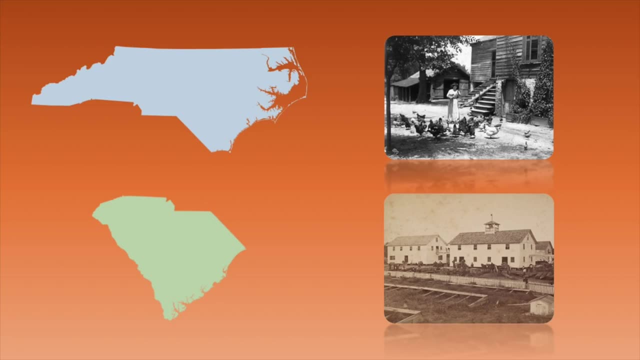 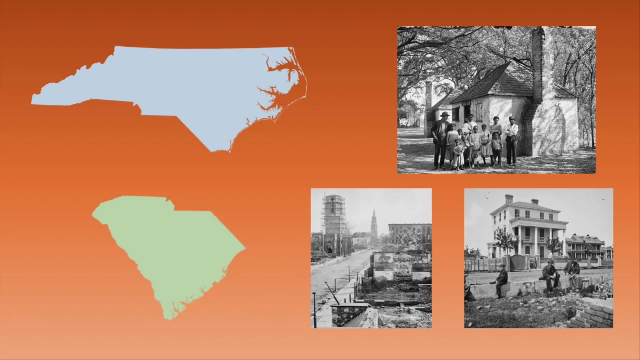 After the Confederates lost the Civil War, both states were readmitted into the Union within days of each other, in July 1864.. Since both states had relied so much on slave labor before the war, their economies now both sucked Now that slavery was illegal. it was an extremely difficult adjustment for everyone involved. After the Reconstruction era, it was the Jim Crow era in both Carolinas, where laws discriminating against blacks and promoting segregation were the norm. The progress that African Americans in the two states made during Reconstruction was halted for decades, until the Civil Rights Movement. 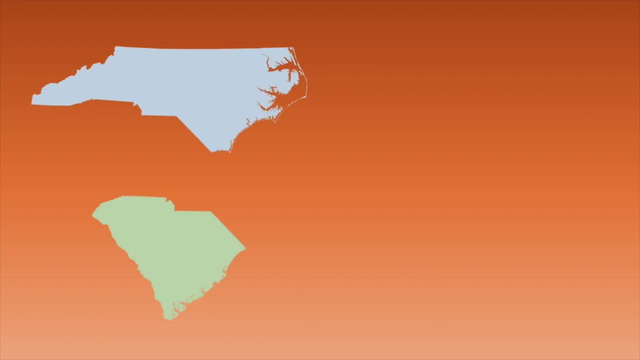 of the 1950s and 1960s, But of the two states, North Carolina seemed to be more of a place where the movement for equality thrived. North Carolina was where the sit-in protests began and where the Student Nonviolent Coordinating Committee was created after all. 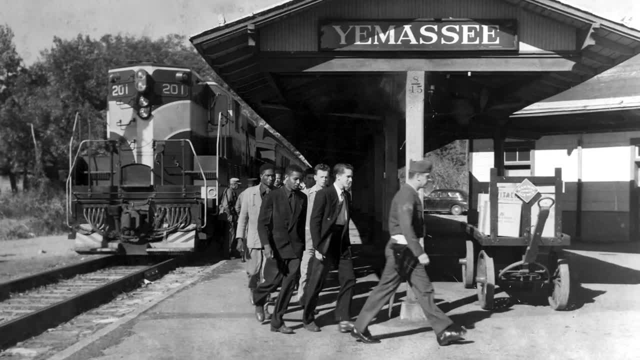 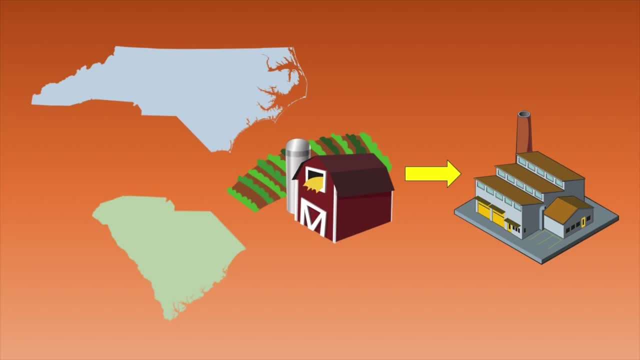 Around. the same time as the Civil Rights Movement, the Carolinas, as well as the rest of the South, finally made the shift from a rural, more agricultural-based economy to a more urban, industrial-based economy. For the first time, there was a shift. Each time, cities started to quickly grow, but mostly in North Carolina. Today, Charlotte, the biggest city in North Carolina, is also one of the fastest growing cities in the country. It had just over 134,000 people in 1950 and has grown to more than 850,000 today. 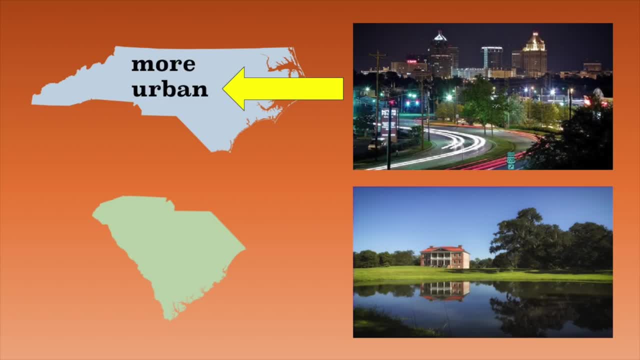 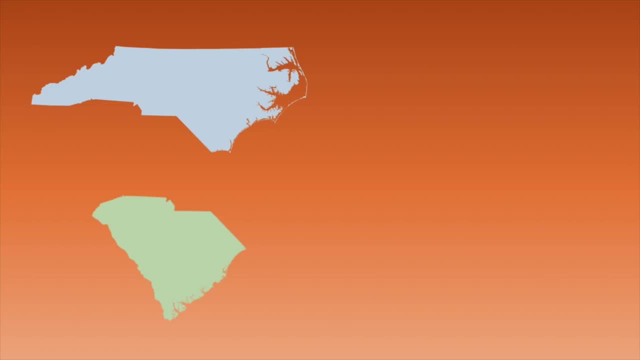 So yeah, today North Carolina is much, much more urban than South Carolina. South Carolina's largest city, Charleston, is also its oldest: It has just 138,000 people. Speaking of population, North Carolina has about twice as many people as South Carolina. 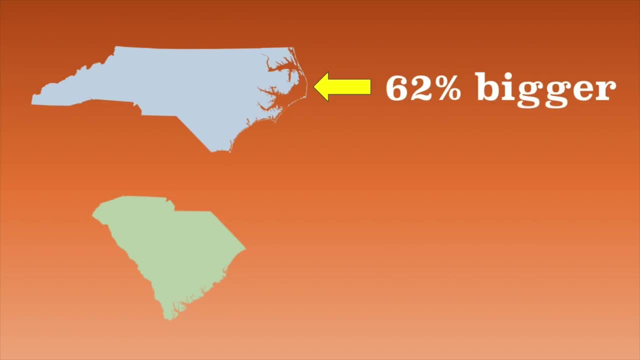 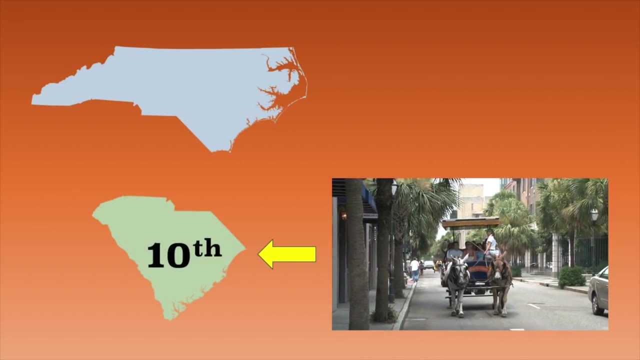 It's not twice as big in terms of actual land, but it's about 62% bigger. It also has more coastline. Sure, South Carolina may be the 10th smallest state, but it's the 24th largest in terms of population. 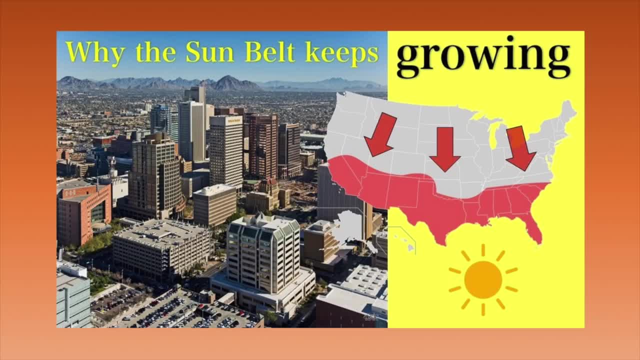 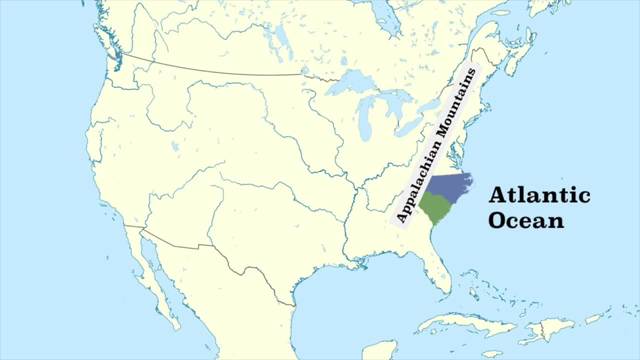 Both states are two of the fastest growing states in the country. Yeah, check out my Sun Belt video if you haven't caught that one yet. Both states border the Atlantic Ocean in the east and Appalachian Mountains in the south. Both states border the Atlantic Ocean in the east and Appalachian Mountains in the south. 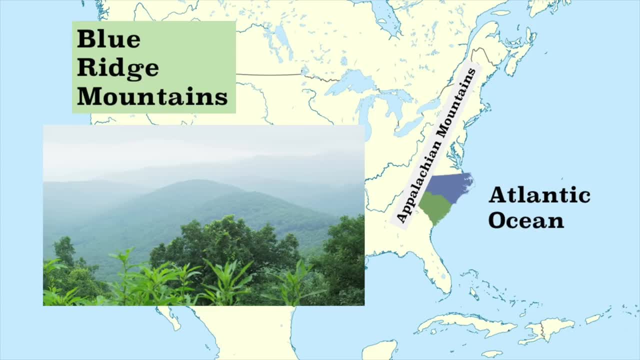 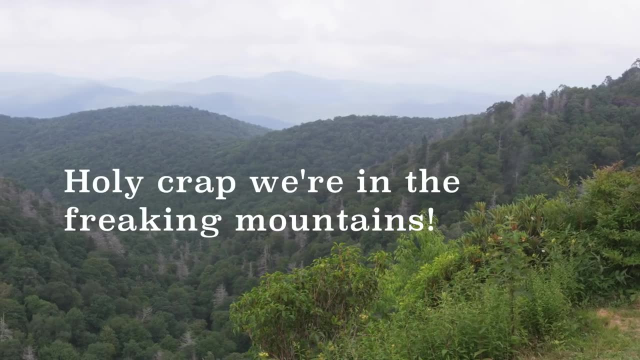 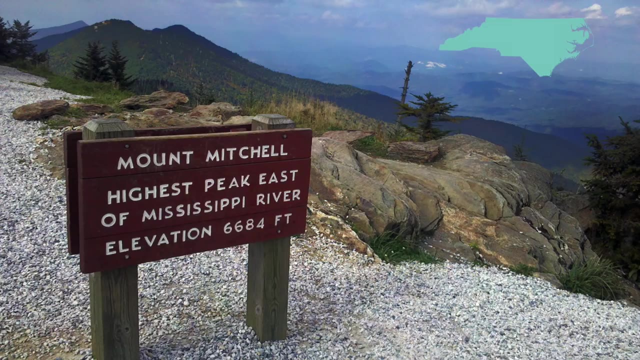 Specifically the Blue Ridge Mountains Driving from the beaches to the western edges of each state. things go from fairly flat and palm trees to gently rolling to HOLY CRAP- WE'RE IN THE FREAKING MOUNTAINS. The mountains are a bit more dramatic in North Carolina, which has the highest peak in the eastern United States, Mount Mitchell. 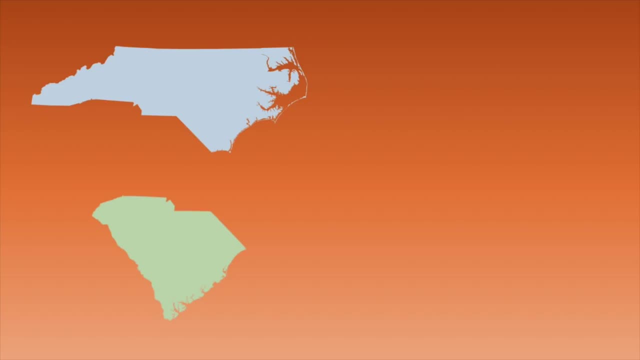 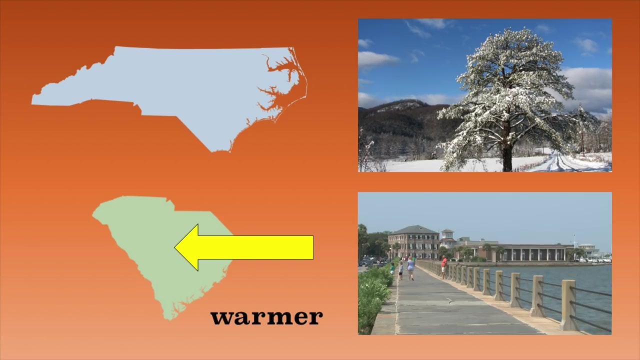 And yeah, since South Carolina is a little bit further, um you know, south, it does have a bit warmer temperatures overall than North Carolina. And yeah, since South Carolina is a little bit further, um you know, a bit milder winters and less snow and ice, but it's not a dramatic difference. And obviously there's the east-west difference. The closer to the coast, the nicer in general. The closer to the mountains, the cooler and less predictable in general. Oh, and the eastern portion of both states has to worry about hurricanes, but the western portion still has to worry about tornadoes. so you know. 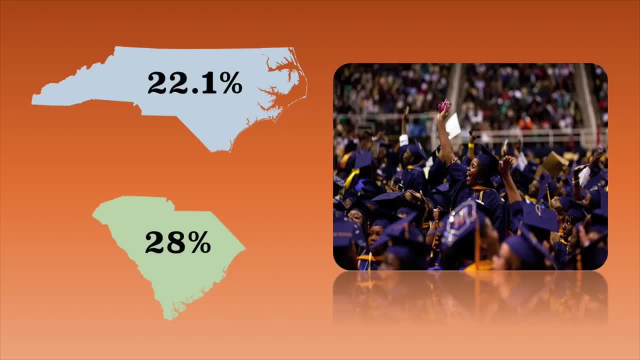 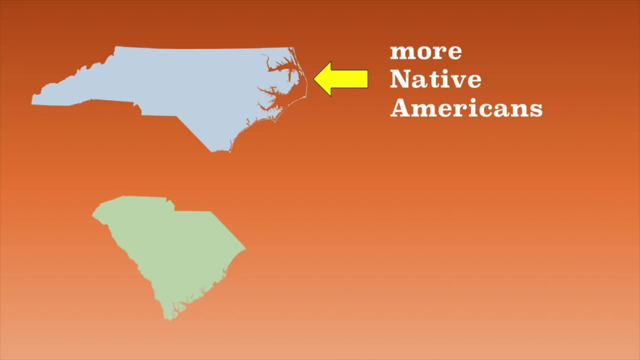 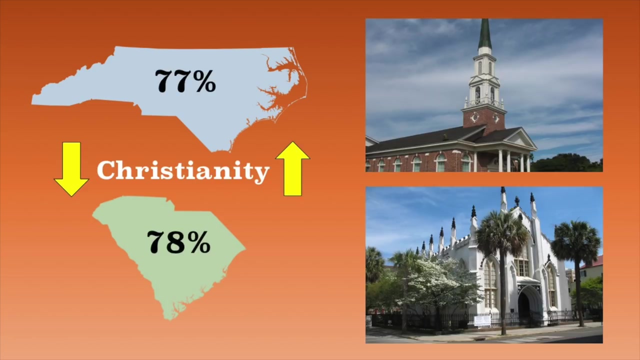 Both states have a really high African American population compared to most other states With a legacy of slavery in both. that certainly makes sense. North Carolina has a much larger Native American presence compared to South Carolina. Both states are pretty religious, with Christianity dominating as the most popular religion in both, Protestant Christianity in particular. In terms of politics, South Carolina is definitely more conservative-leaning. North Carolina has become a swing state for presidential elections in recent years, while South Carolina hasn't voted for a Democratic candidate since 1976. And that's only because it was Jimmy Carter who was the governor of Georgia, their next door neighbor. 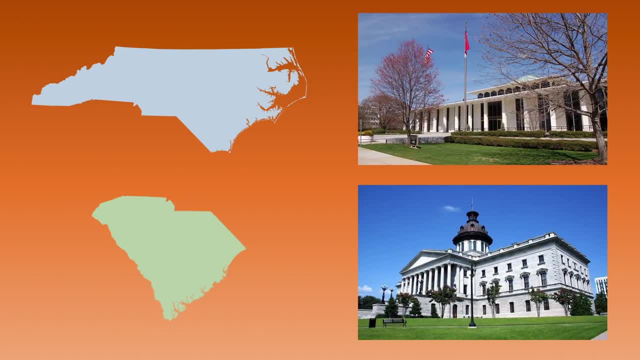 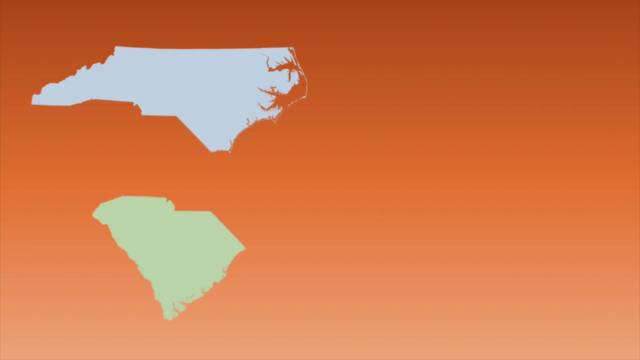 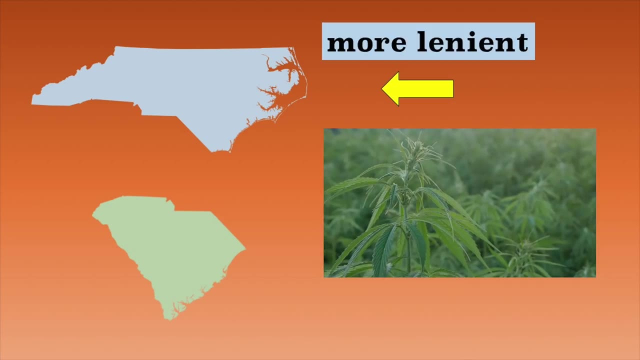 Both state legislatures are majority Republican. however, The North Carolina General Assembly and South Carolina General Assembly are pretty dang similar. Some state laws are noticeably different in the two states. The fireworks laws are much more lenient in South Carolina. North Carolina has decriminalized marijuana use and possession a bit and will most likely legalize it before South Carolina does. 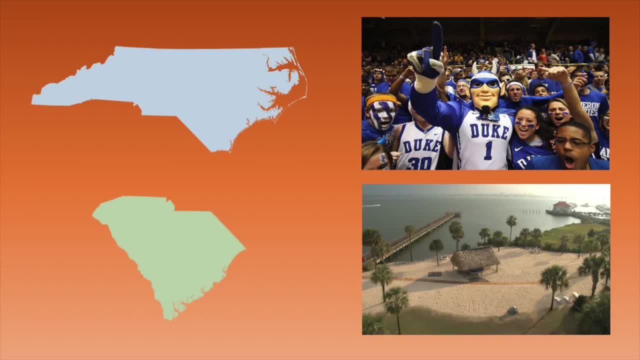 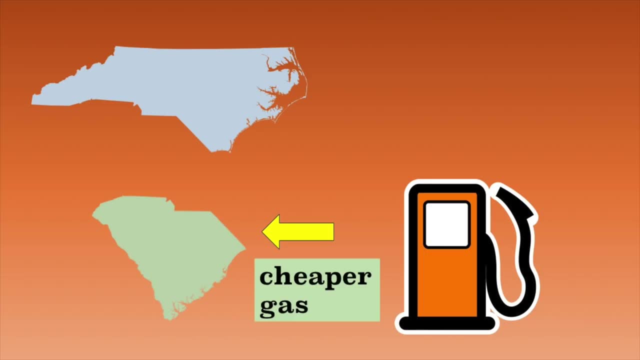 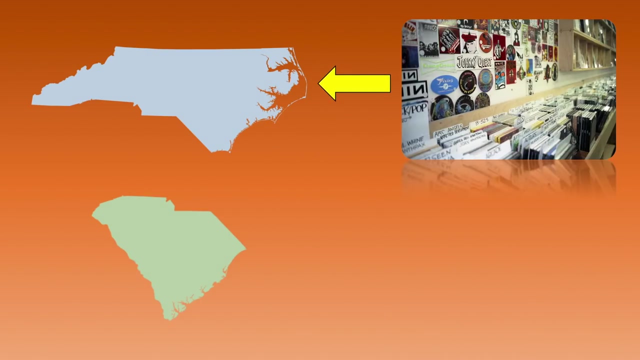 Although it was really difficult to research taxes in both states, I've determined South Carolina has a lower tax burden overall. The most noticeable difference is that gas is cheaper in South Carolina due to a smaller gas tax. Sales taxes start lower in North Carolina compared to South Carolina, but counties and cities often add their own sales taxes on top of it. 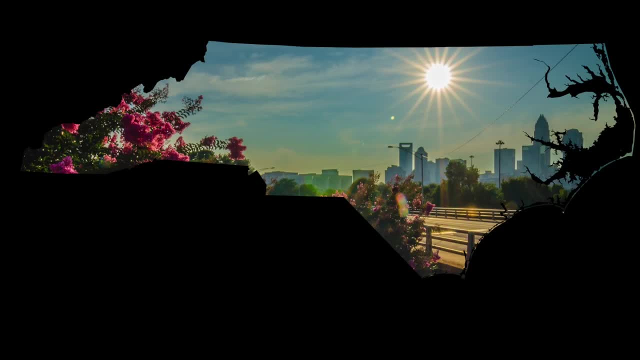 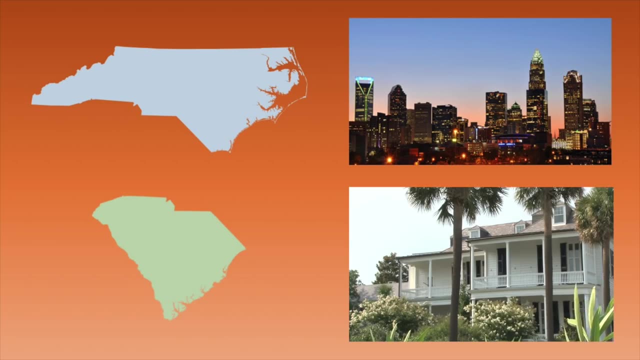 North Carolina seems to have a more promising economic future compared to South Carolina. According to Forbes Magazine, it's the number one state for new business, But both are rocking with similar unemployment rates and job growth rates. Both states have identical poverty rates. 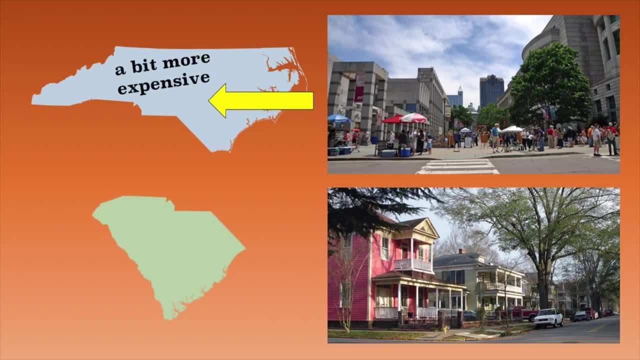 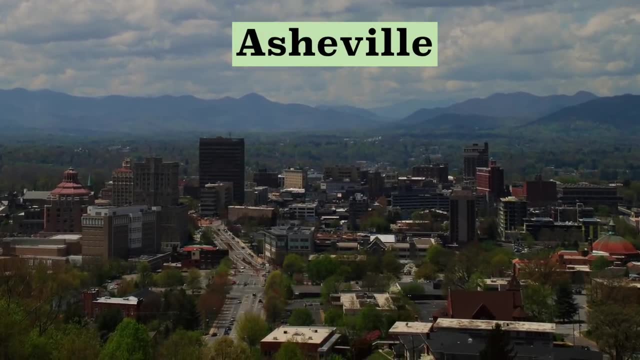 The cost of living is pretty similar too, although it's slightly more expensive in North Carolina, especially if you move to Asheville. What the heck Asheville, I mean? are you really that cool Speaking of poverty? South Carolina has higher crime overall. 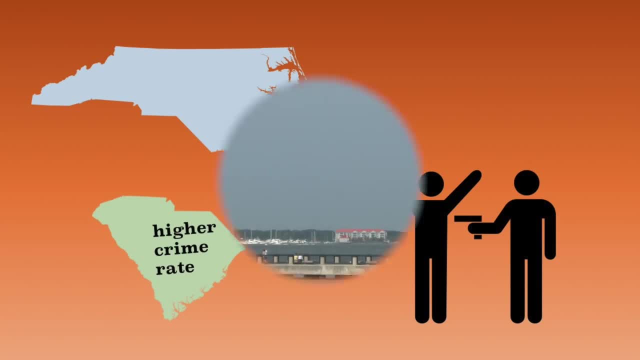 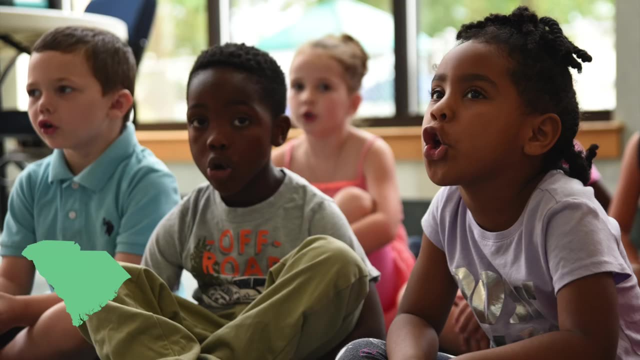 I'm sorry South Carolina government about publishing that and stuff, But South Carolina gets three more sunny days. It's a crazy year compared to North Carolina. Did that make up for it? South Carolina also spends more money per student on education, But that doesn't match up with the crime statistics. 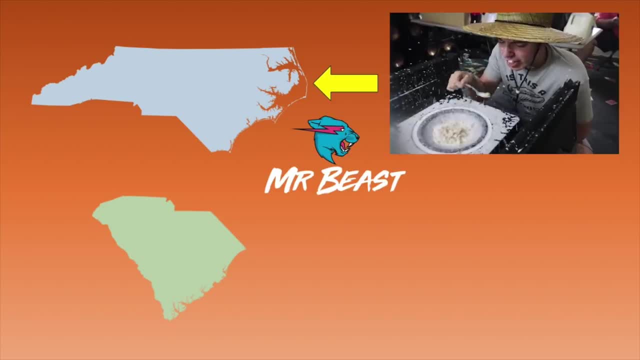 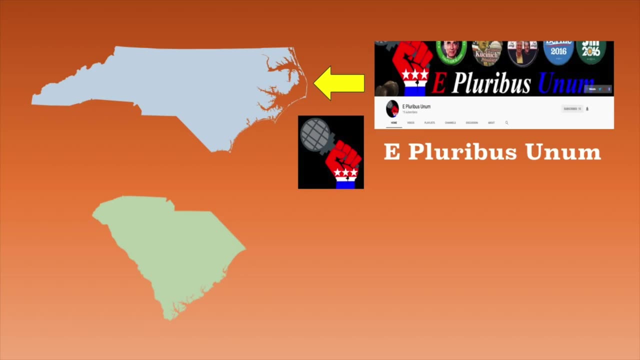 Hmm, Let's see What else. Mr Beast is from North Carolina- That's not his real name and no, I am not related- And Fernando from the YouTube channel E Pluribus Unum is also from North Carolina. Ian is from South Carolina.